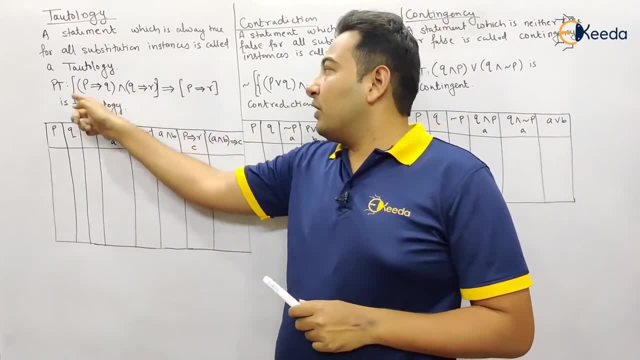 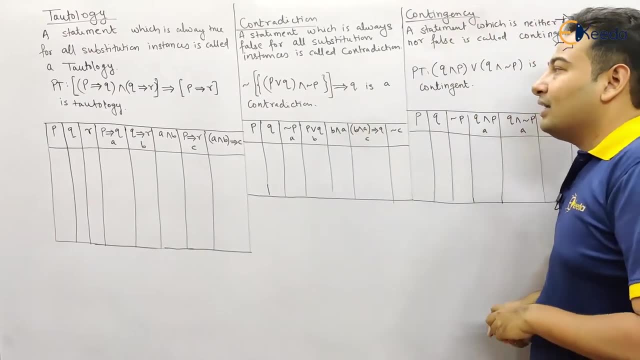 That means after finding the value of this particular statement. that means this particular column. if all the values are true, then it is called tautology. What about contradiction? After finding the value of this particular statement? that means this particular column. 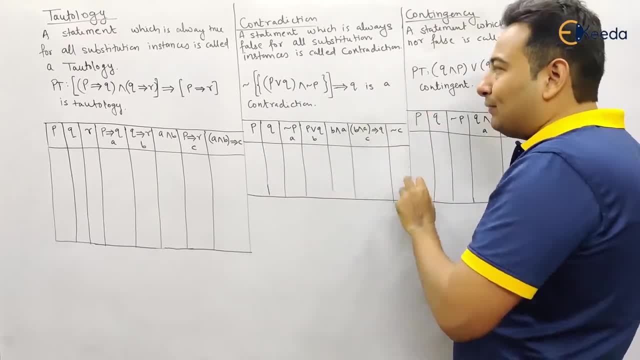 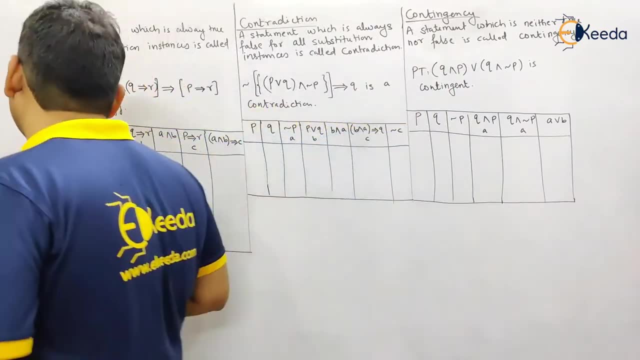 if all the values are false, then this column, then it is contradiction. and if we get mixed values- true and false mix- then it becomes contingency. Very simple to prove. Let us start. First of all, we need to prove this. 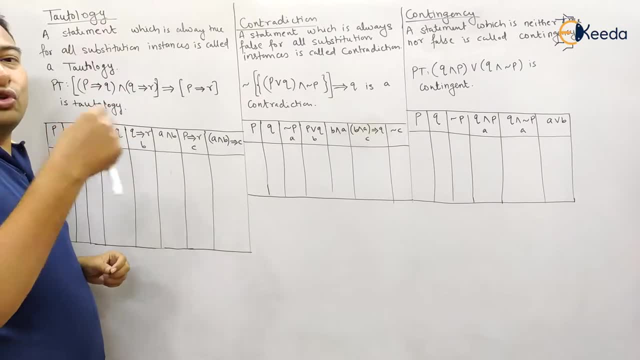 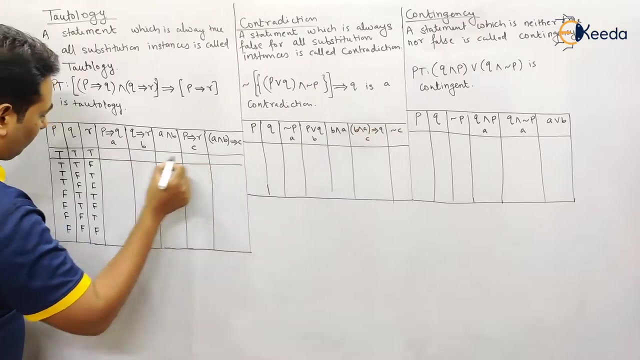 Here there are three terms: P, Q and R. So therefore two cube. that is eight possibilities. Therefore, first four true and then four false. What next? Two true, two false And finally it will be alternate true- false. Let me draw this line so that there will be no confusion. 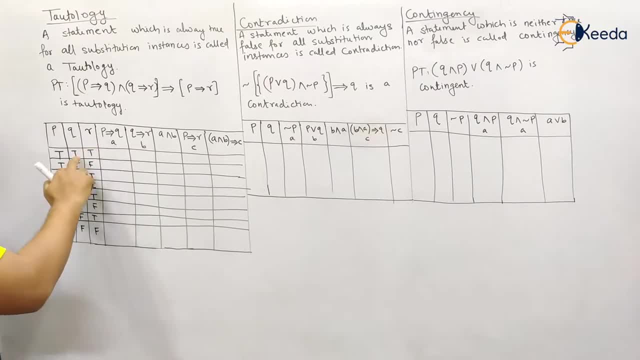 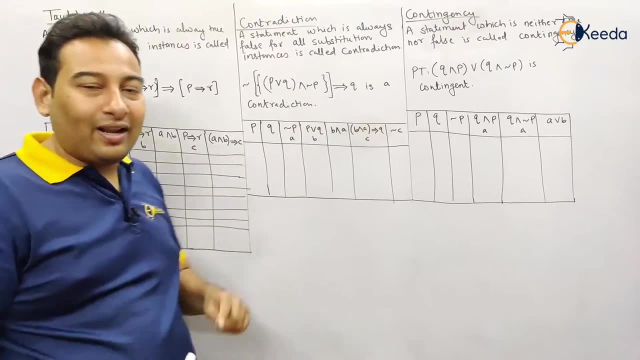 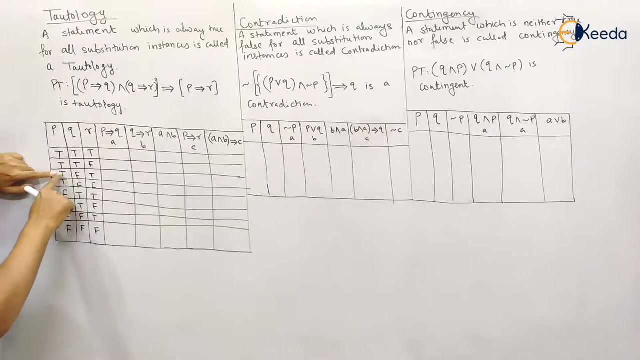 So let us start See. the first is P implies Q. So that means we need to look at these two columns. and implies means what? Remember the trick of implies false? That means TF, that is false. So let us check. See here: TF, so that is false. 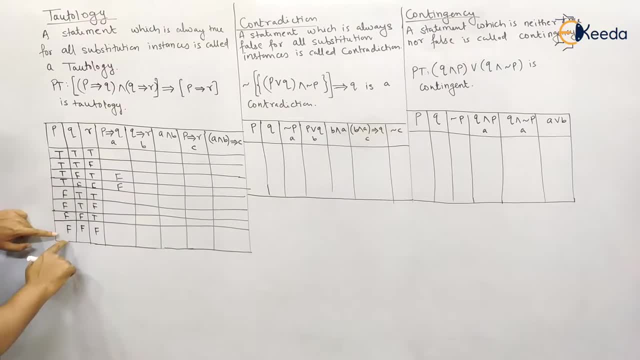 Next: again we got TF false. That's it Only two instances we getting TF, so that is false. Rest, everything is true. We got P implies Q. Next, Q implies R. Again, we need to check tough. See: here we got TF. then it is false. 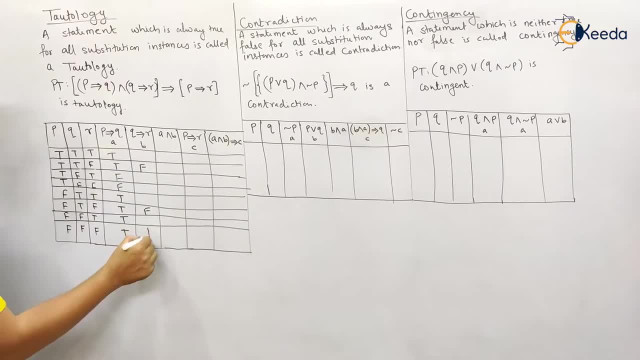 Here we have TF, then it is false. Rest all the instances will be true. Next, A and B. For simplicity or for convenience, you can say: we have assumed this is A and this is B, So we need to prove this. 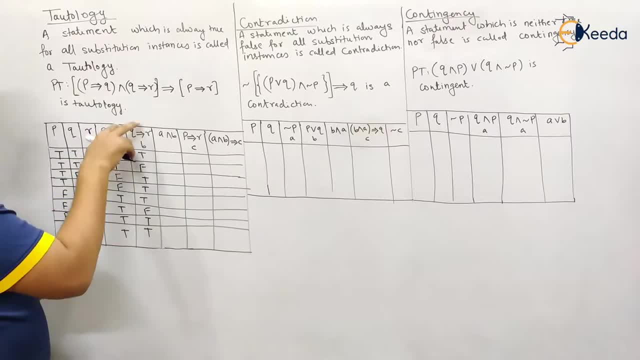 We need to find it out A and B. So conjunction of these two statements and true and true is always true. See here, both are true. Therefore it is true. Next, see here again, we getting both true, then it is true. 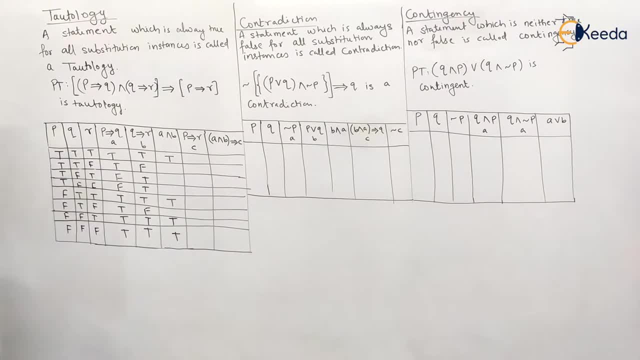 Here also, we getting both true, Here also we getting both true. So both true, true Again. both true Again. both true and both true. Rest, everything will be false. Let's move on. P implies R. So what is P? 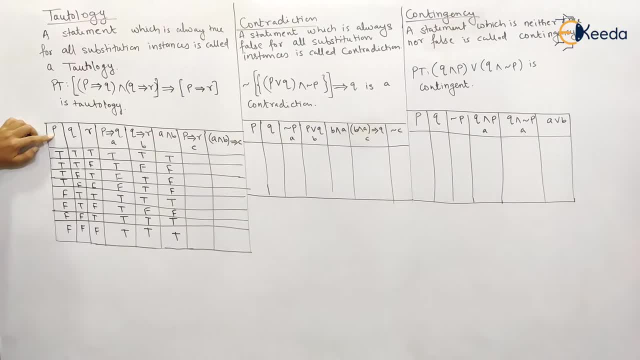 P is this. P implies R. that means this. So P implies R. We need to check tough because it is implies. So if it is TF, then it is false. See here it is false. Next, see here it's false. 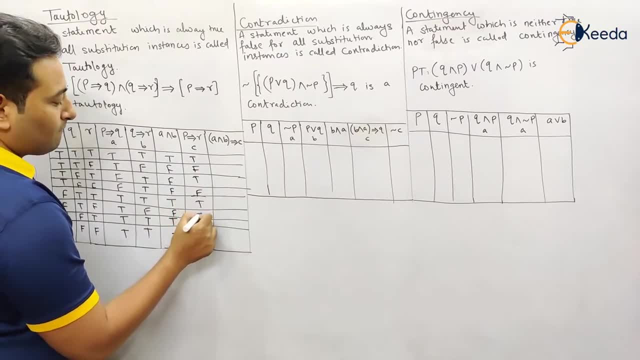 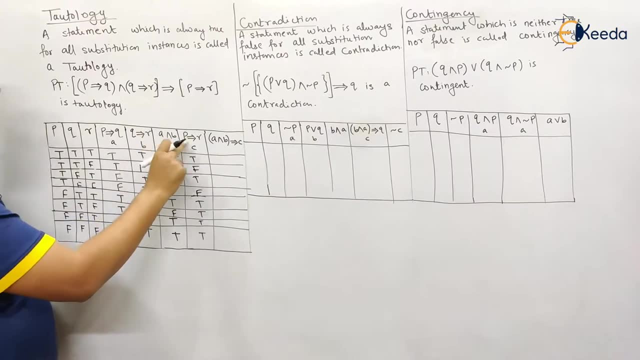 That's it. Rest everything will be true. And finally, we have A and B implies C, So this is C, A and B implies C. So wherever we get tough, that is false. Rest everything is true. Now let us check. 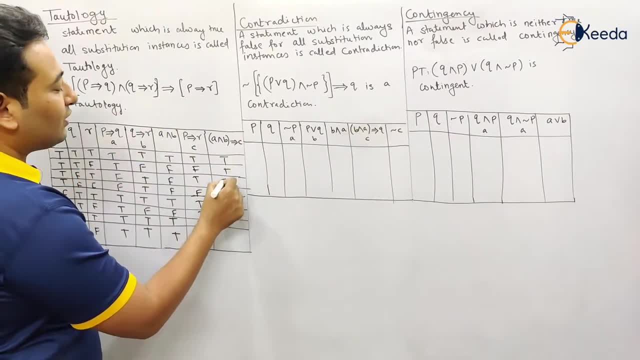 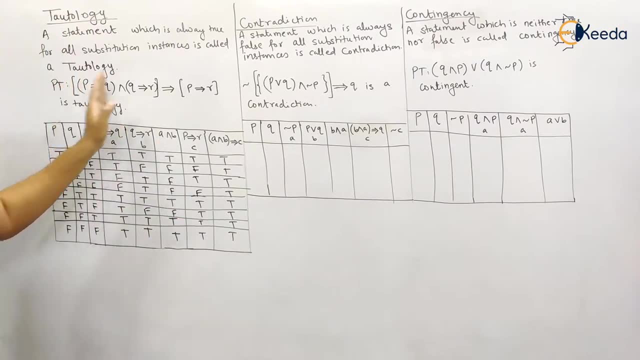 Nowhere we getting tough. That means all the instances are true, All the values are true. See here what is a tautology statement? If the statement value is true for all the instances, then it is a tautology. Therefore you can say it's a tautology. 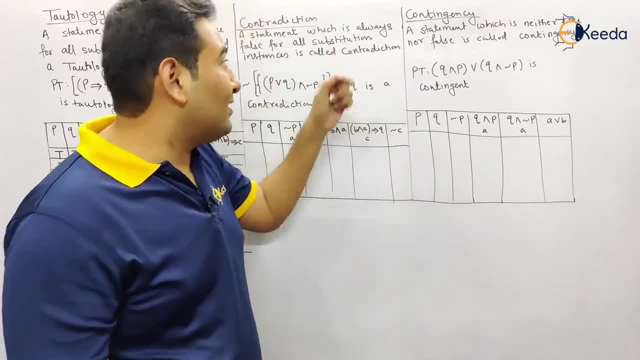 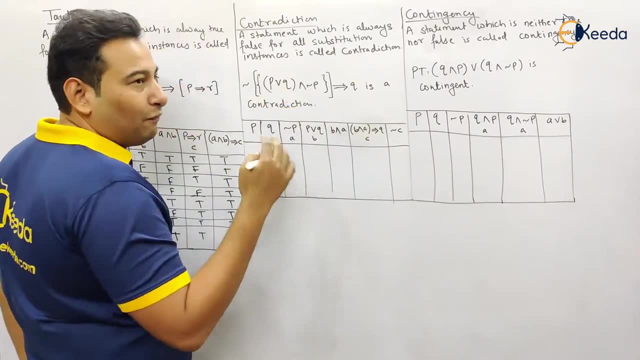 Since we all got true values, then it is tautology. Next is contradiction. That means we should get all the false values. So let us start Here. there are since only two values: P and Q. therefore, 2 raised to 2, that is four. 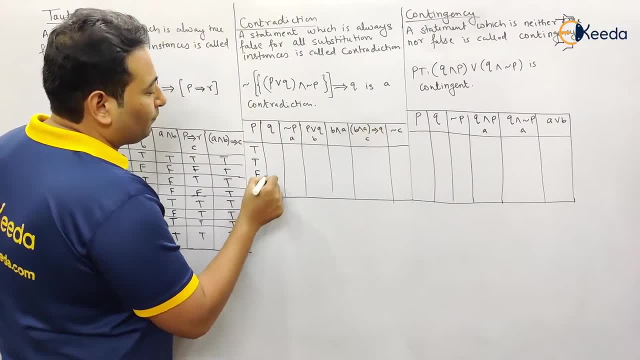 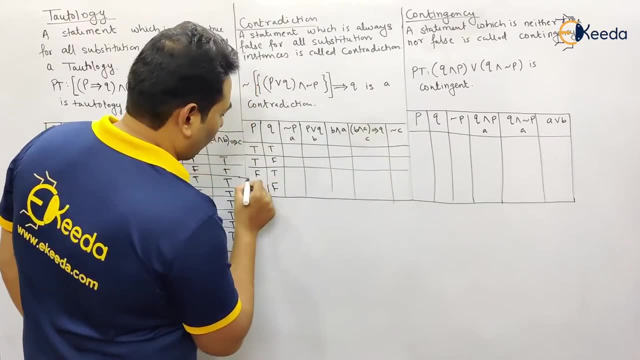 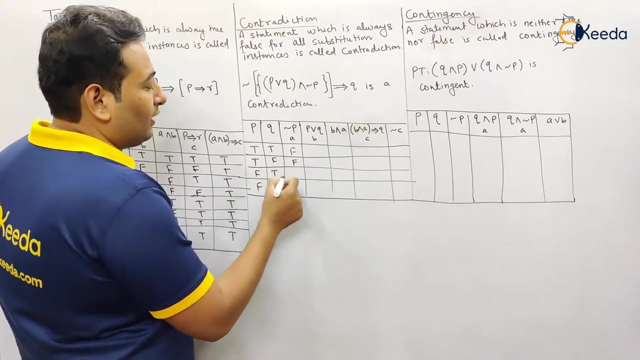 So four possibilities: true, true, false, false. Then true, false, true, false. What next We need to find? negation of P. So negation is true. negation of this term: true, negation is false. and this is true. what next? p or q. so this is your. 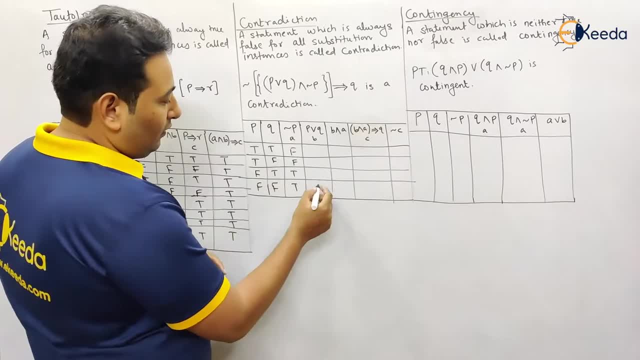 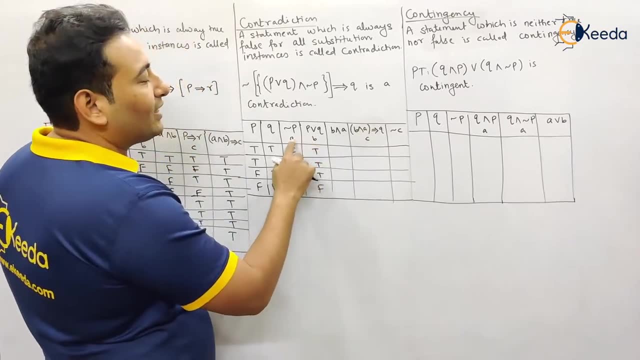 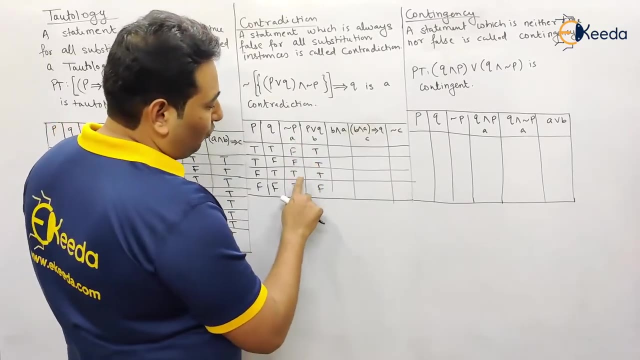 disjunction: false or false is always false. c here, both are false, then it is false. rest: everything is true. what next? b and a. so we need to take intersection. uh, we need to take conjunction of these two. that means true and true is always true. so c here true and true is always true. rest: 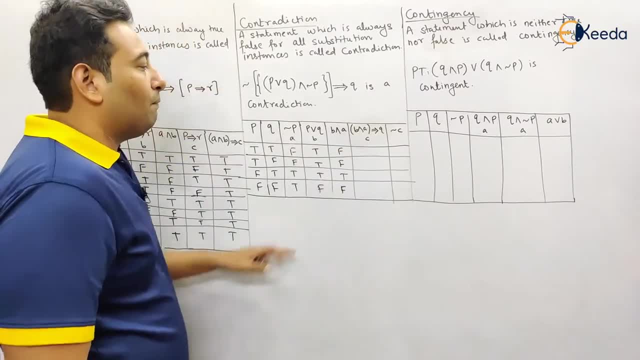 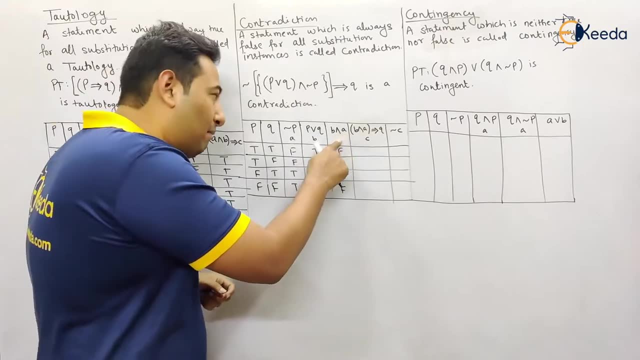 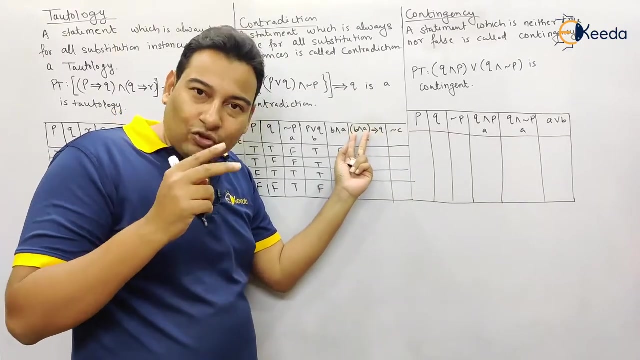 everything is false. let us move on. b and a- we already got it- implies q. that means: from this, we need to check this. so b and a implies q- you cannot check q implies this: there is a difference. b and a implies q. that means first you need to check this column, then you need to check this. 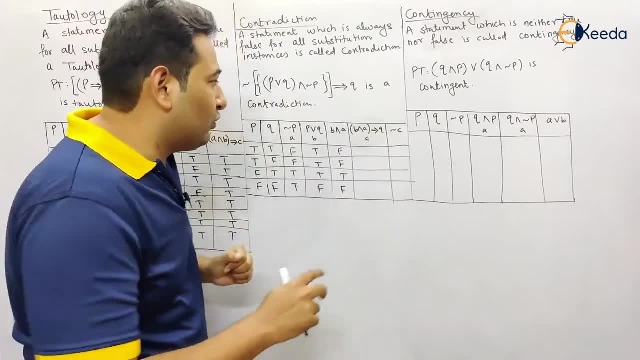 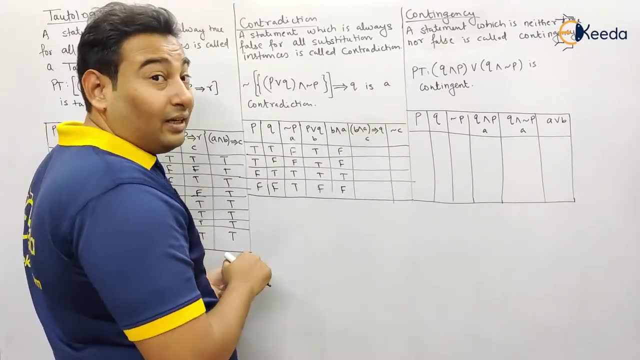 column if you take in a reverse order. that is not allowed. so first of all we're going to check this and then this q. so from this to this we need to take, we need to check tough. that means true here, false here, c here, true here, true here, nothing. so there is no combination of 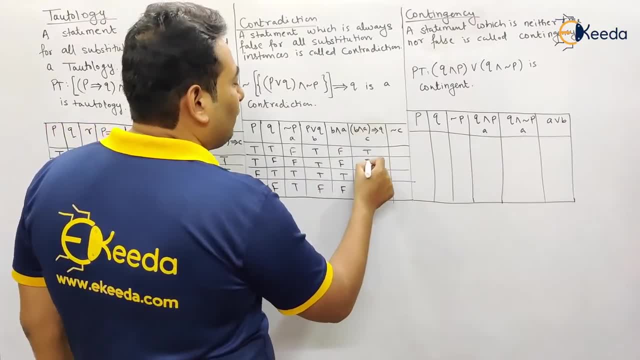 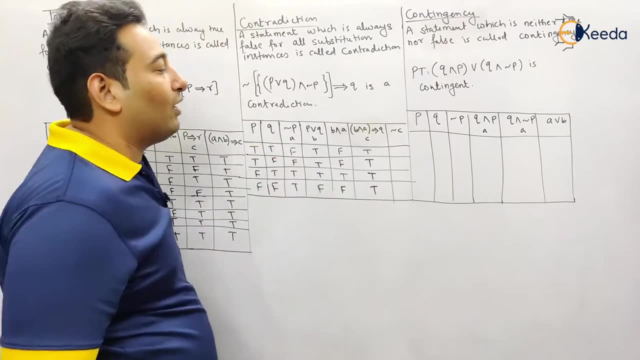 tough, true, false, we are not getting. that means all are true, because if we get true, if we get tough, then it is false. we are not getting tough. t from here and f from here. we are not getting. therefore, all are true. what about negation of c? that means you just need to take the negation of. 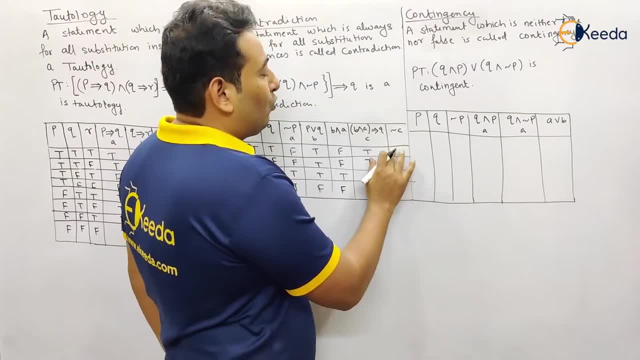 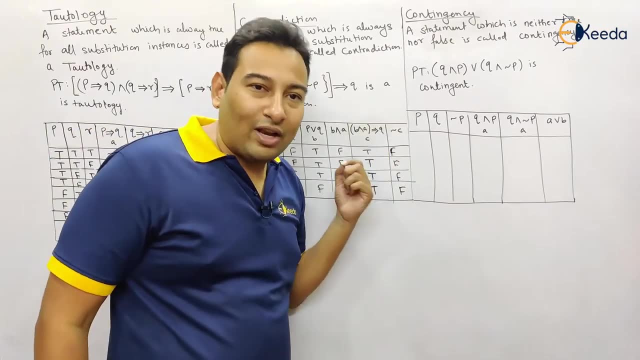 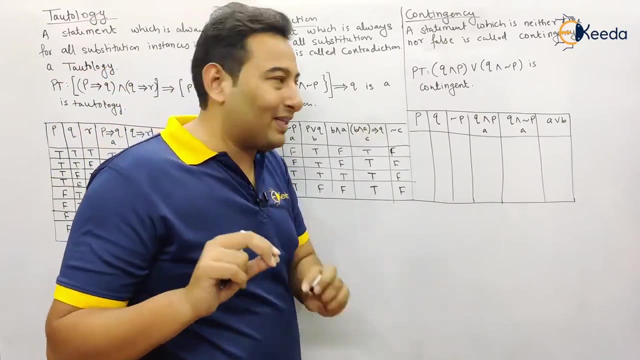 it of this column. so that is what true negation is false. this is false, this is false and this is false. that's it. it is contradiction, since all the instances, values are false. therefore, it is contradiction. what is next? contingency? it means what? mixed? true and false, mixed a statement which is neither tautology nor contradiction. 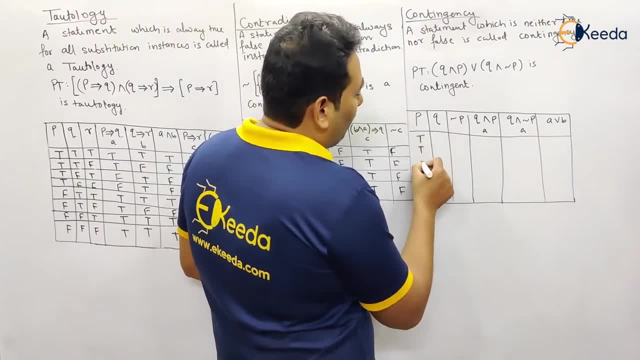 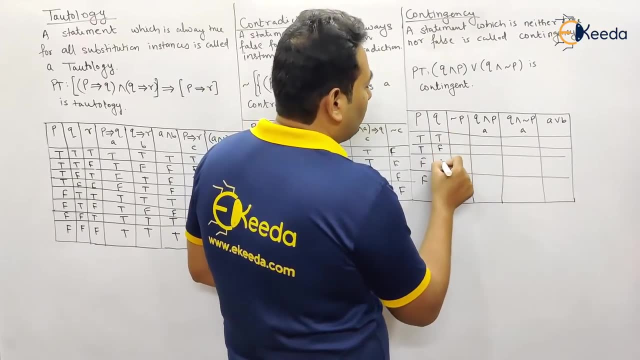 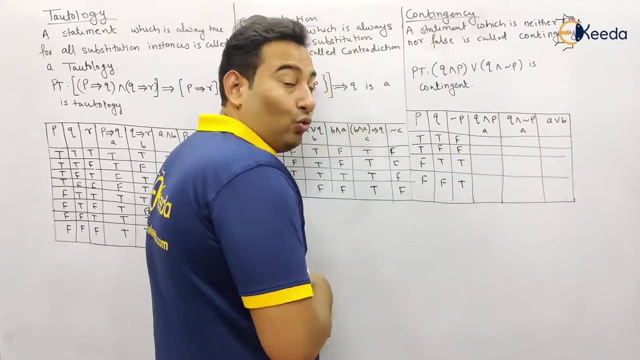 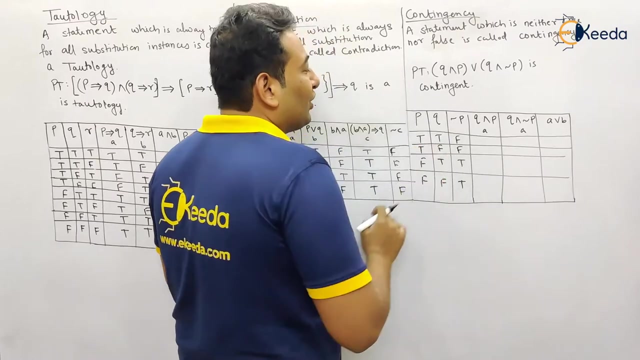 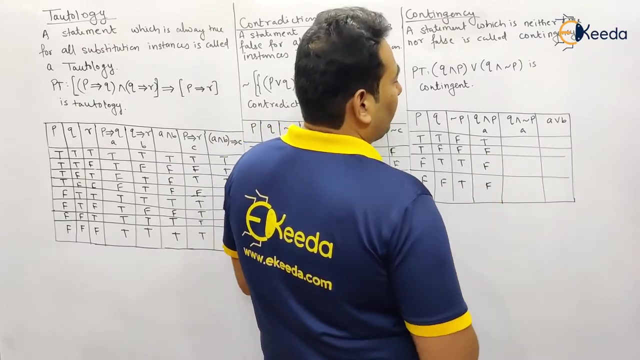 becomes contingency. let us start: true, true, false, false, true, false, true, false. next negation: p. that means this will become false, false, true and true. q and p. so q and p, we need to take its conjunction. that means both are true. then it is true, true and true is always true. rest: everything is false. what next? q and negation of p. that means we need 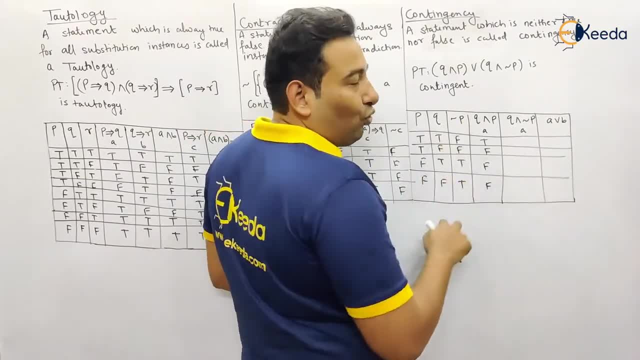 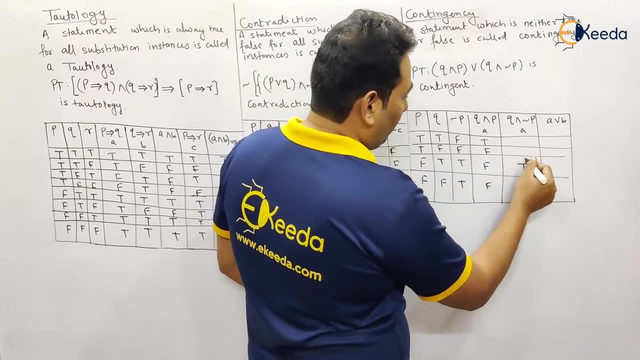 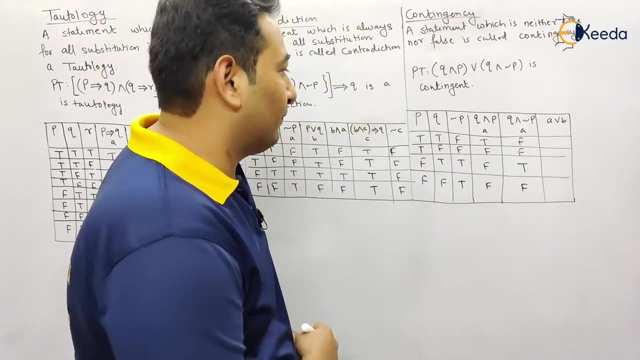 to find it out, this q and negation p. so between these two columns, we need to find it out. and that means true and true is always true between these two columns. so see here: true and true is always true. rest, everything is false. finally, a or b. so this is the a statement, this is b. that means 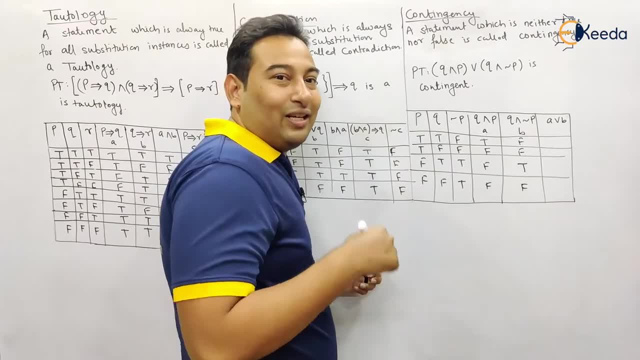 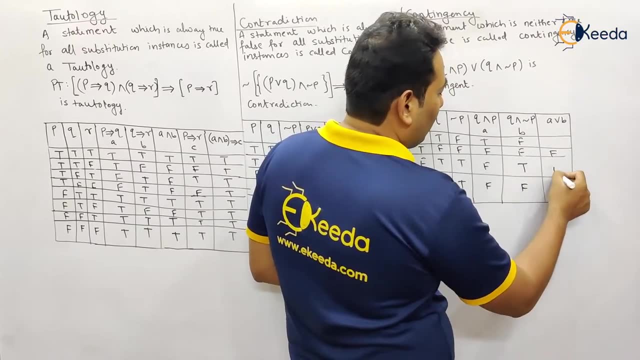 between these two statements. we need to check this junction. that is, or false or false is always a false. see false or false is always false. false or false is always false. this is true, and this is true now if you check this particular column or you check the instances of this particular.